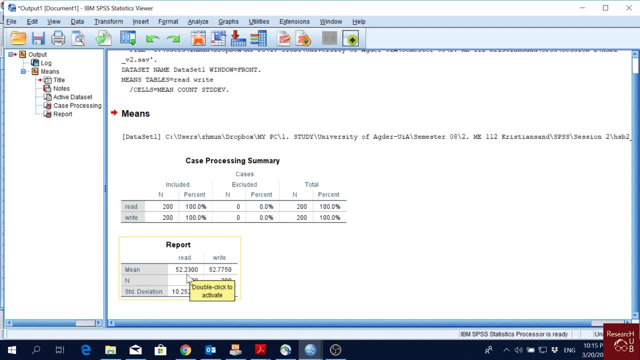 two groups. so mean of reading a score is 52.23 and writing is 52.77. we can have many groups, as many groups as possible, as many groups as we want, and here we see we have the n is 200 number of observations and we have no missing values and we also see the standard deviations here. so that's it. 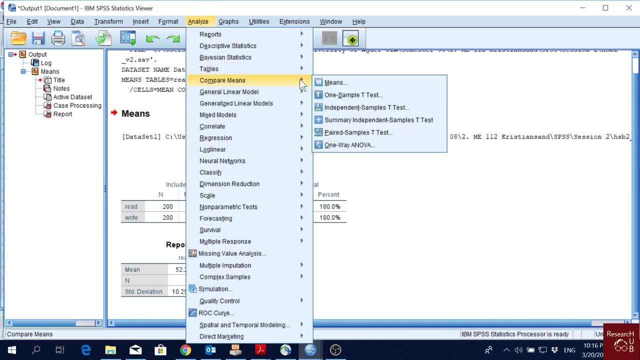 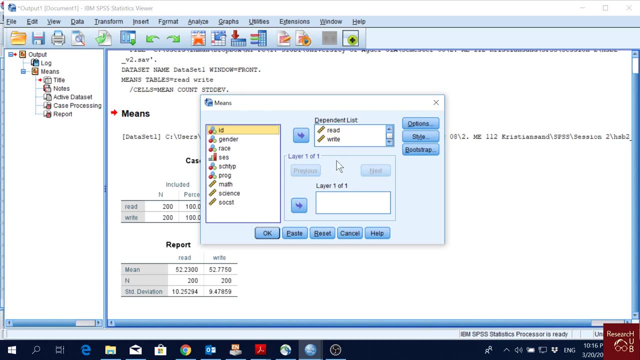 actually we get from means in in the means option. we have another option here. you can see layer one, so we can actually categorize the mean of different variables. for a categorical variable, for instance, if i pick gender in layer one, then i will see the mean of male and female for these two. 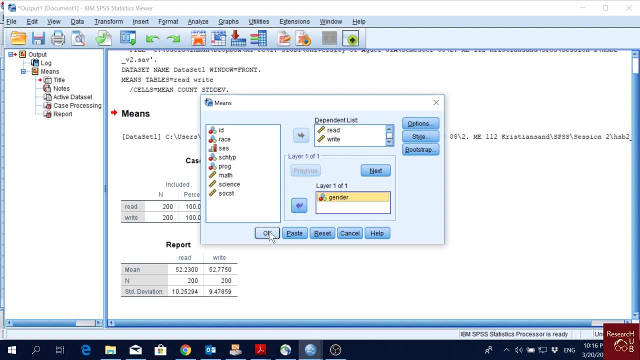 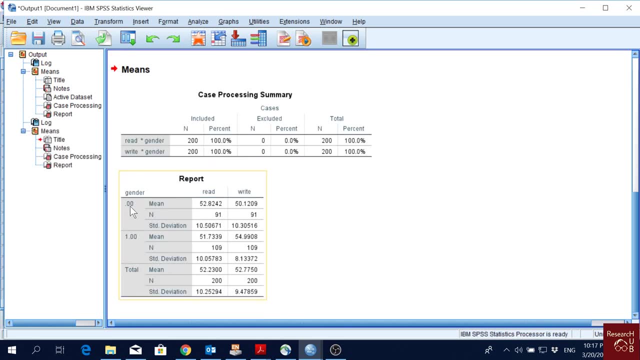 re for for these two variables here. okay, so let's have a look. how does it work? i will click ok, simply, and here, as you see, i have the gender uh in. in my case, uh, zero was male and one is female, so i dummy coded them and i'm going to pick gender, and i'm going to pick gender, and i'm going to pick gender. 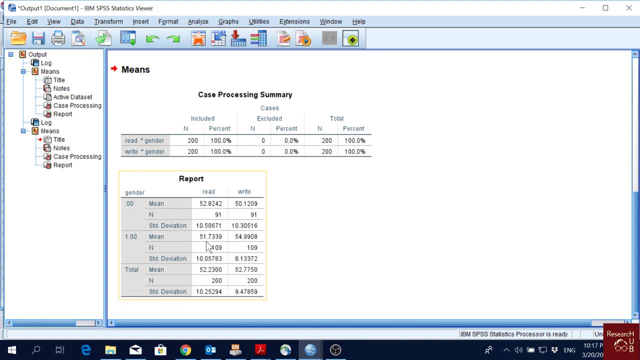 and there are means for reading and writing and again the means for female in in reading and writing. so and we also see the number of observations in in male group and female group. so in male we have 91, in female we have 109, and we also see the standard deviations in both, in 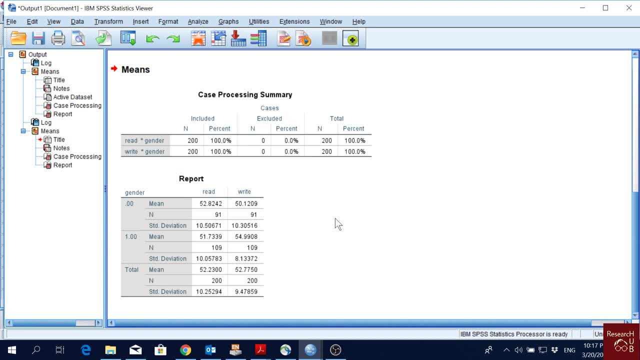 both cases and the total score as well. so that's what we get from the only mean option. but maybe we are not really. maybe we are not really interested only in checking the means. but we want to see if there is a significant difference among the two groups. we want to do some hypothesis testing. 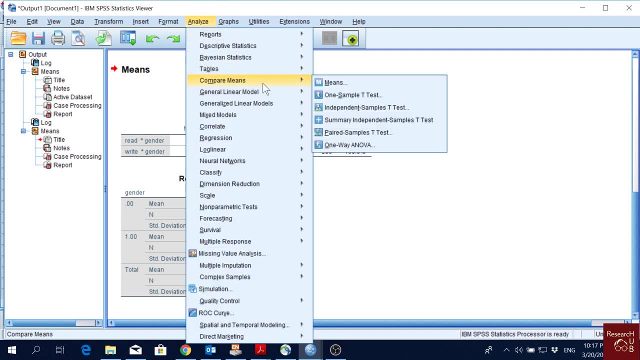 or maybe let's- let's go through one by one. so let's go to the one sample t test. so when we use one sample t test, we use one sample t test. when we want to compare mean of one group of people with a hypothesized number, okay, mean. 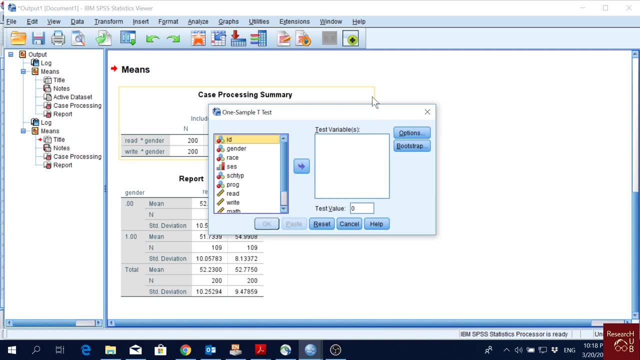 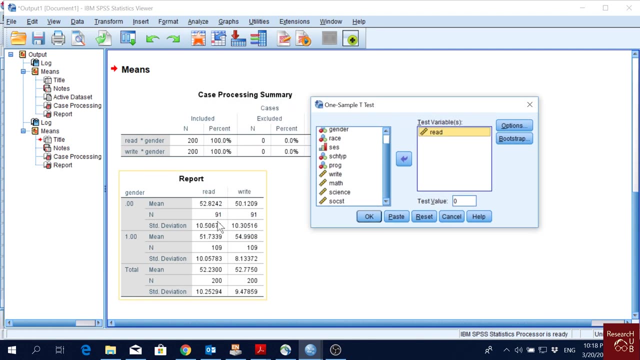 let's see: uh, i'm going to click one sample t test. so let's say i pick reading a score here as my test variable. so the reading score mean is approximately 52. right, as we have seen before here we can see: uh, reading a score is, yeah, about 52.. but let's say we normally see that in these. 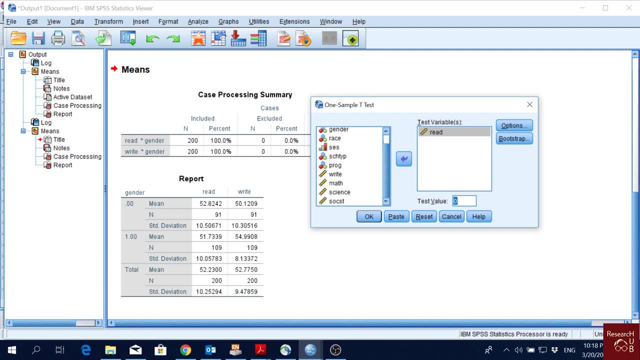 kind of exams. people normally score 60, but in our case people are scoring 52. but is 52 significantly from 60.? when we consider for the standard deviation and the distribution of the data, is it significantly different from 60 or not? that's what we want to see. we have a hypothesis. 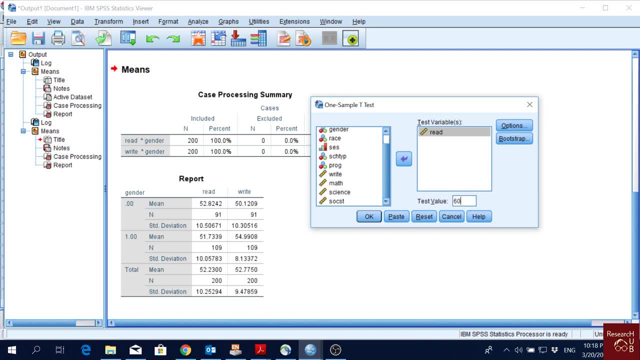 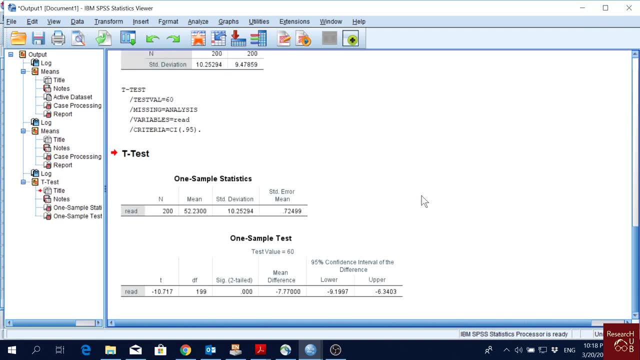 number in our mind and that's when we use this one sample t test. so i'm just gonna put the hypothesis number here and i will click ok. so this is the output we get. we have 200 observation mean and a standard deviation of my independent variable. here we see the t test score: ttd. 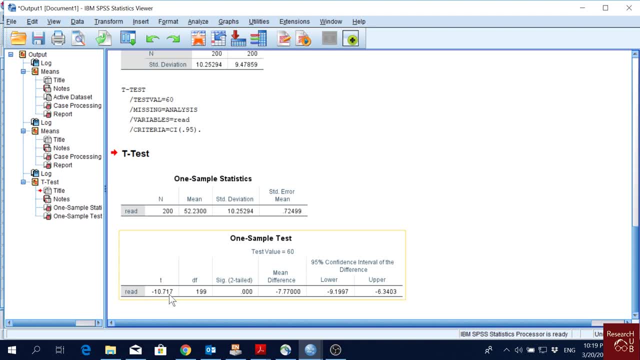 score. it's a minus 10.71 which is way high than minus uh. 1.96, high way extreme, then minus 1.96. normally the t score, i think uh for two tail tests like here, where we do not know the right when, where. 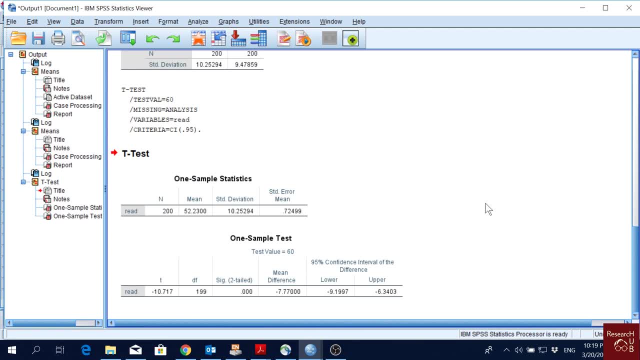 we do not know the direction and normally we would uh have a value of 1.96 for statistical significance of 0.05 at 5.5 percent statistical significance. so it's it's a much extreme than that. that means there is significant difference in the values, in in the mean score of reading and in the value of 60.. 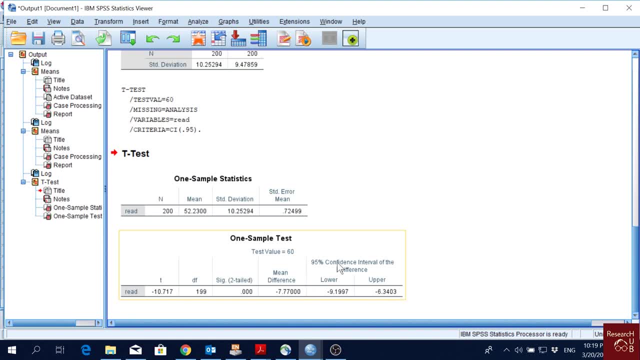 and the difference is here minus 7.77. we also have a confidence interval here. the lower confidence interval is minus 9 and upper is minus 6.34. so it's it's a confidence interval for the difference. so the difference is here, but the lower limit is 9 minus 9.19 and the higher limit is minus 6.34. okay, 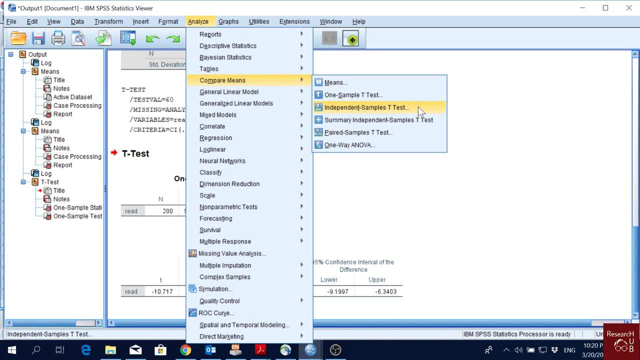 so now again we go to mean we have another type, independent sample t-test. so when do we use this? when we want to compare means of two groups- okay, two different groups. that's when we can use this independent sample t-test. let's have a look. so let's say, i pick again the 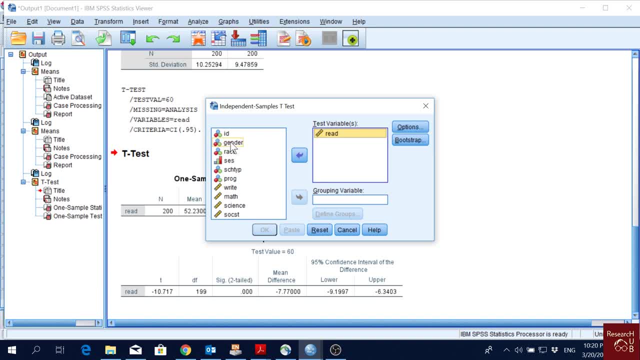 score. so in this categorical variables we have gender. in gender we have two categories, so we can maybe use that as a grouping variable. we have also pro- i think we have any school type. we also have two categories, so we could have used that as well, but we cannot use this race. 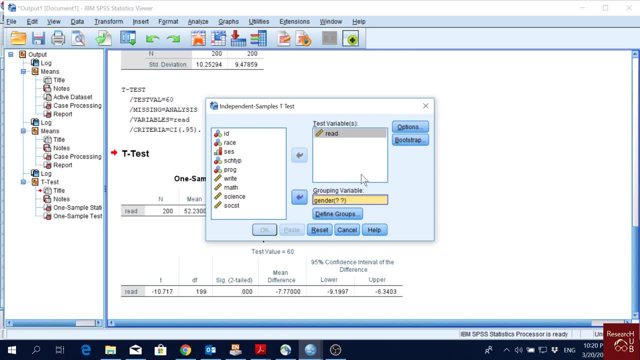 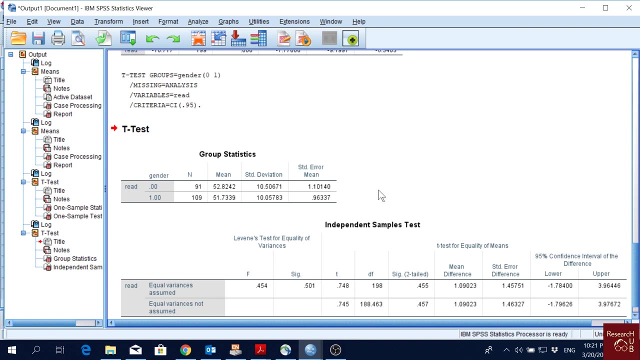 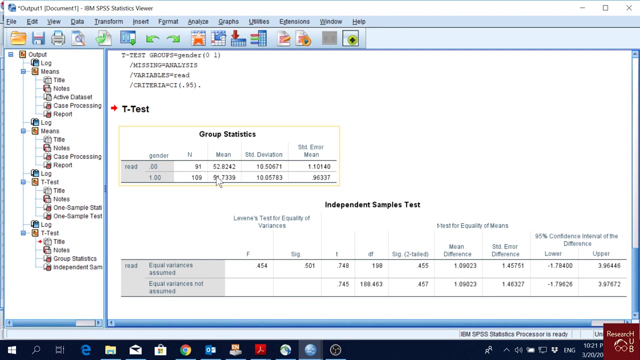 ses or program, because there we have more than two categories. so independent, independent sample t-test is only for two categories. okay, so we have to define the categories zero, and zero is for male and one is for female. continue, and okay, so we get this result. so what do we actually have here? here we have some summary: in total we have 200 and we have 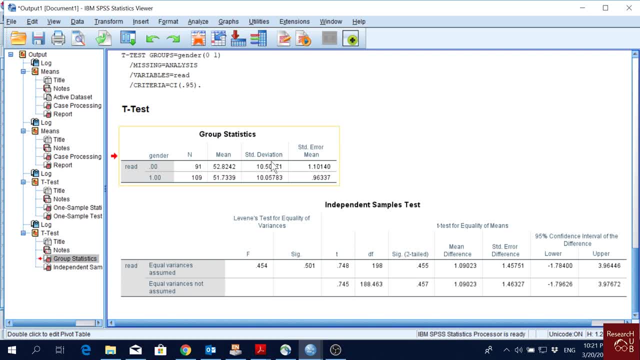 91 male and 109 female and their means, their standard deviation and their standard error. so when we look here in the independent simple t-test results here actually what we first get is Linnaeus test for equality of variance. so for when we do mean comparisons of 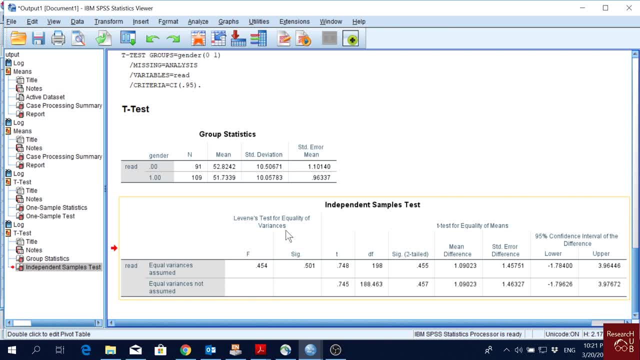 different groups. there we have this assumption that the variances of the different groups should be equal, and that's what we get here from the Linnaeus test for equality of variance test, which is done by default by SPSS, and in this test the null hypothesis is that that the variances are equal across. 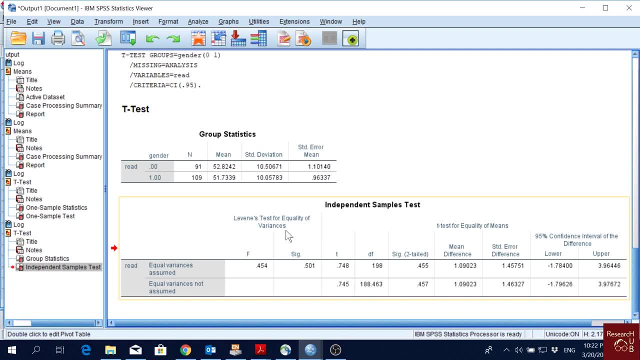 groups. an alternative hypothesis is that the variances are not equal across group. okay, so, as we see, the significance value here is higher than 0.05. so we fail to reject the null hypothesis. so we go for the null hypothesis because we cannot reject it. so the null hypothesis is that that variances are equal across group. so 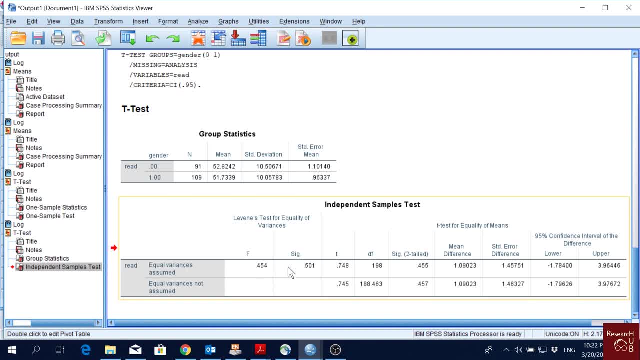 when our equal variances are assumed, then we will look into the first row of the results. if our significance value here was not uh, was was less than 0.05 and our null hypothesis was rejected, then we would go for this row. then we would go for the second row where when equal variances are not assumed, but in this case this: 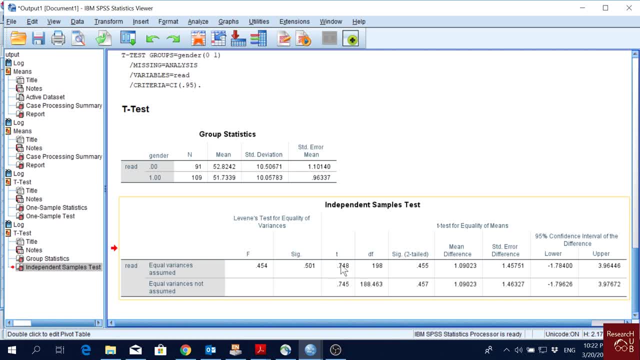 is not the case. so we can actually look into the first row. okay, so now from here we have the real result for the independent sample t test. so first f, f statistic and significance value, that's for the lennox test for equality. and then we come here in the test for equality. so we see the t. 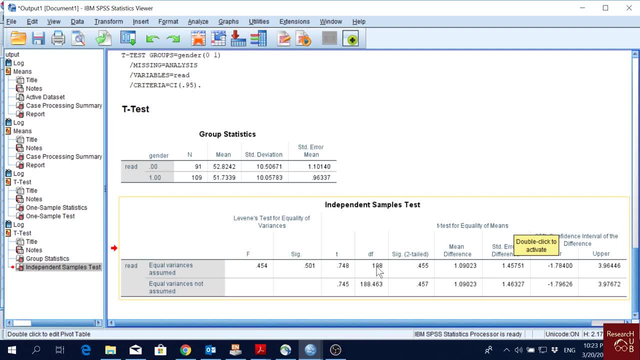 value is actually quite low and as we have two groups, so degrees of freedom is the whole sample minus two. so that's why we have my uh 198 and as the t score is quite low, which is quite low than 1.96, as i said before, like normally for um, for, for, for, 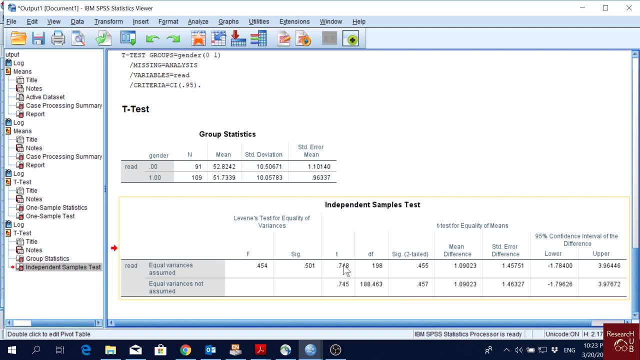 two-tail test. uh, we would expect values of t-score higher than minus 1.96- or plus 1.96- uh, extreme than plus or minus 1.96- to get a significant value at a statistical significance of five percent, but which we did not get here. so that's why we do not have a significant 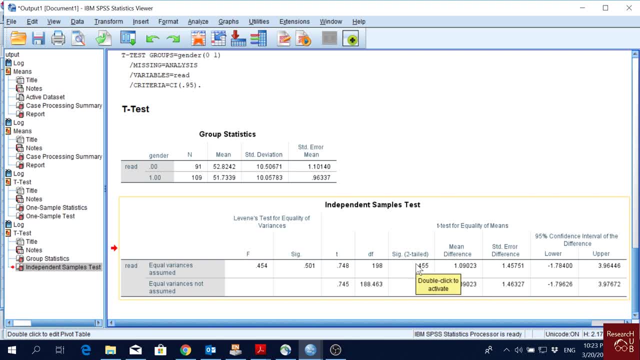 difference among the uh, among the two groups here. so from here we can conclude that there is no significant difference in the reading score of the major and female students and accordingly we have the mean difference here and standard error and lower and upper limits for the main difference. okay, so 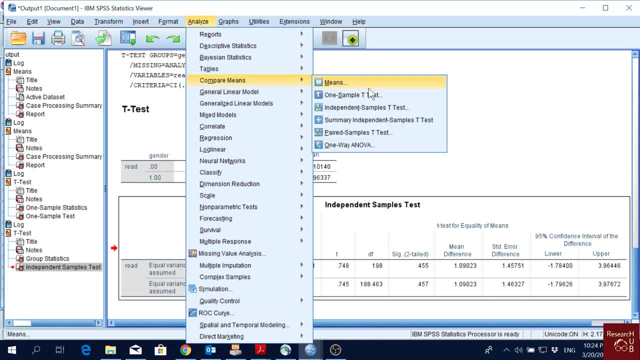 that's it for this part. but then let's say we want to see difference among more than two groups. what can we do on those cases? we have to go for one way and over when we, when we want to compare the means of more than two groups, it could. 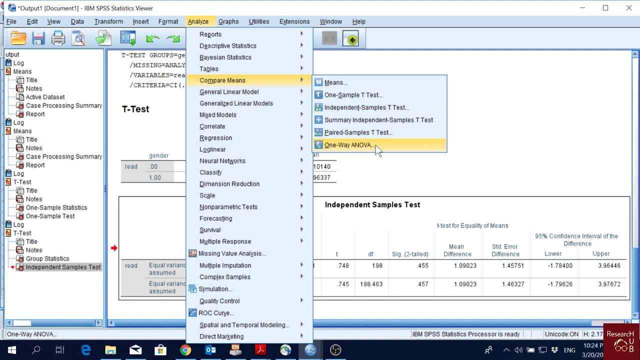 be three, it could be five, it could be any, any groups, any number of groups more than more than three. okay, maybe I would not compare ten groups, but like three, four, five, six, that's fine. okay, so in those cases we'll go for one way over. so 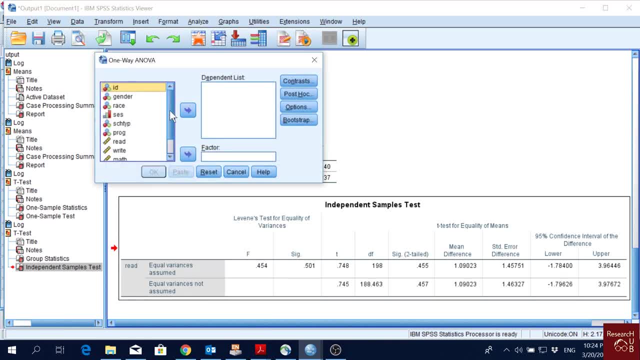 let's click here and see how it looks like. so we'll just. we first have to drag the dependent variable here and let's say which one. let's say, we pick the program. in program we have three categories: vocational, academic and general. so we will pick that. 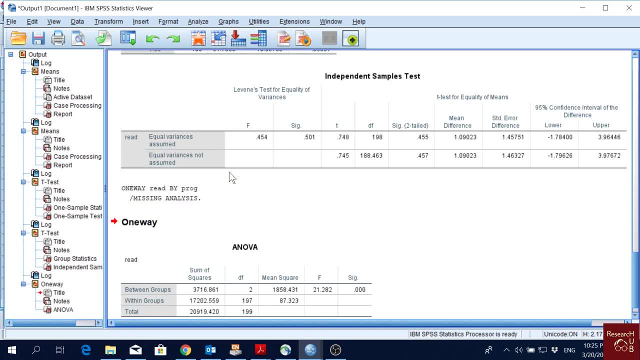 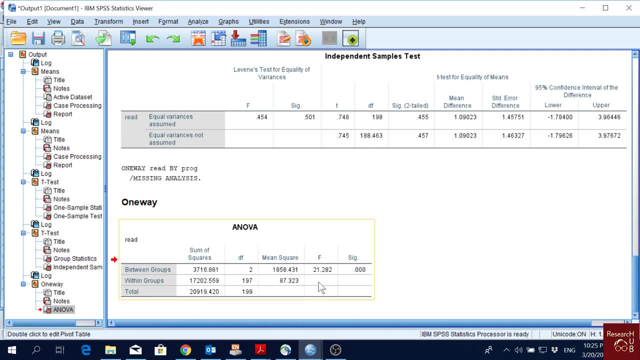 as a factor. okay, and we'll click OK. so now we get the result for ANOVA. okay, so we have the sum of squares, degrees of freedom, mean of squares, every, statistics and significance. so we see that significance is very high. but we have to remember one thing: when we have ANOVA: 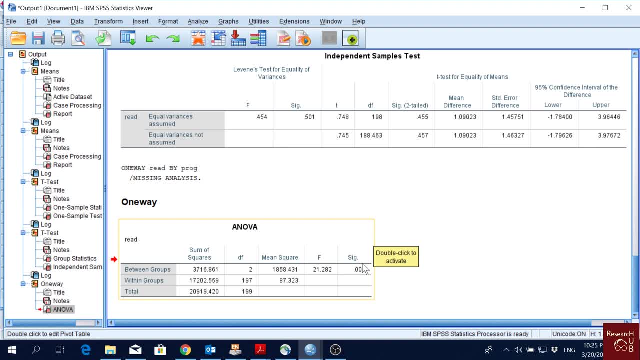 results. the interpretation of the significance value here is that there is a significance value difference between at least two of the groups in our data. so we we have more than three group, more than two groups. so in in in this case we had three groups, so we have significant difference between. 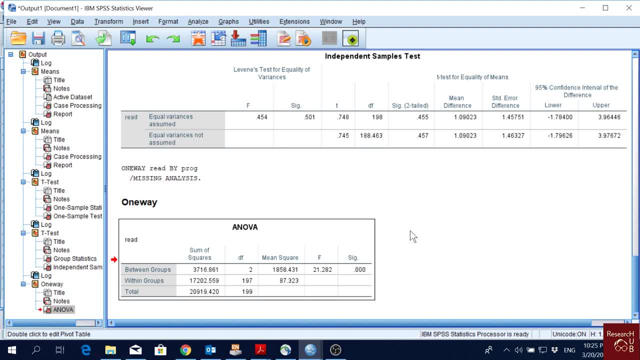 at least one of the groups, one of the two groups. it could be in all of them. there is a significant difference, but it may not be the case. maybe it's only one group where maybe there is a significant difference among only one group or between only one group. so may not be among all of them, but 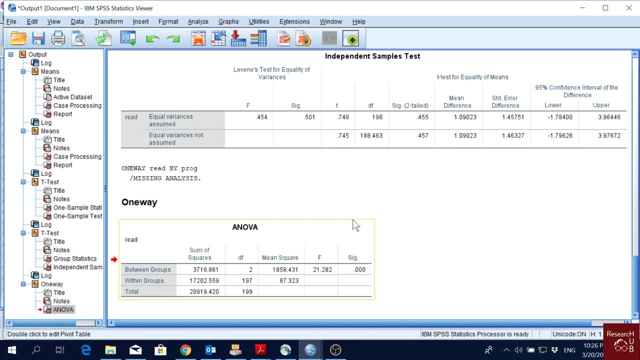 could be also among all of them. okay. so that's, that's the situation. so here we see that, okay, there is significant difference, uh, between the groups here, but then maybe we're interested to see actually among which groups there is a significant difference. so in this case we will. 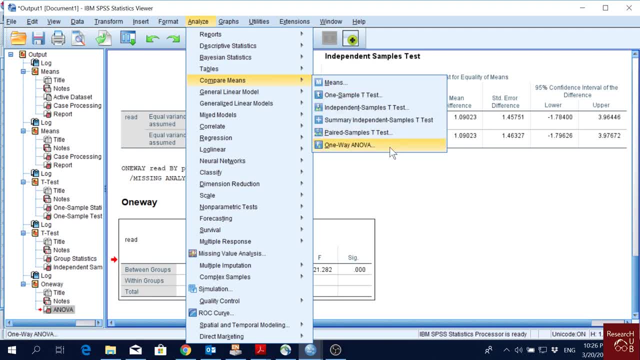 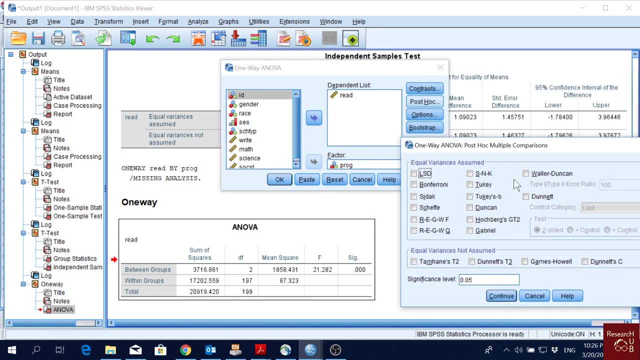 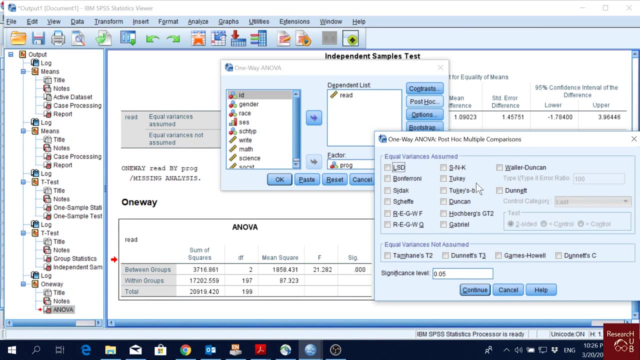 get again. we'll go again to analyze, we'll go to compare mints one way and over so we can do some post hoc test to see this. i'll go for this. so here, uh, we have two options: equality of variance assumed, equality of variance not assumed. so most of the cases maybe we will assume equality of variance. let's say we assume. 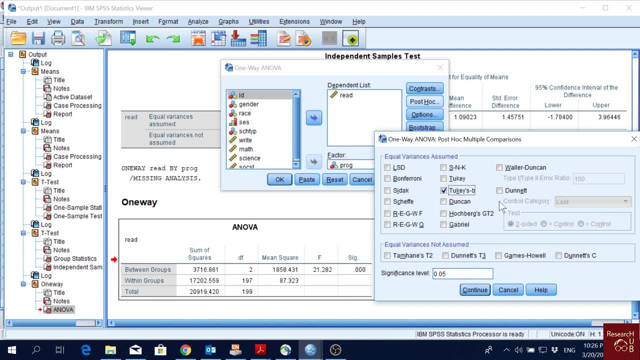 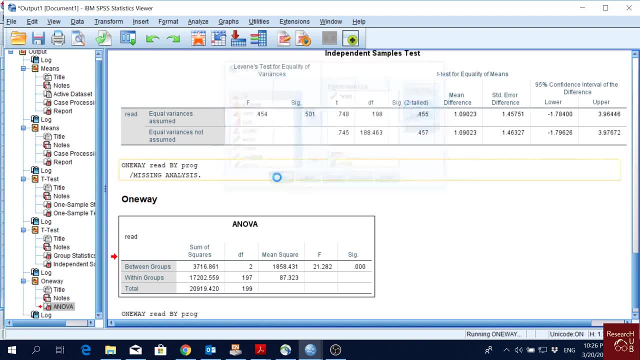 equality of variance and i'm picking this one, takis b. this is one of the most common one, so i'm just going to click continue and i'm setting my significance at five percent level. i'll click continue and okay. so this is the result i get. so here: subset: 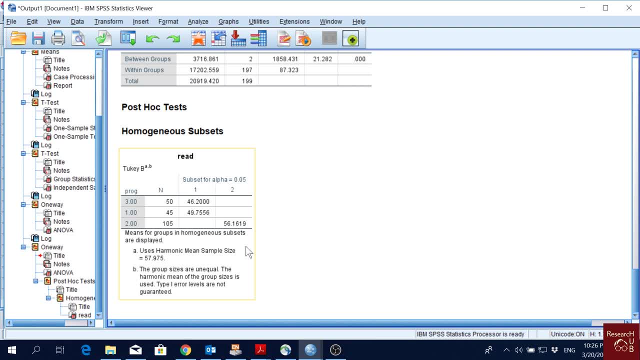 for alpha 0.05. so we have two groups, homogeneous subsets. so in the first group we see that group three and one are together. this means that at five percent statistical significance there is no significant difference between the group one and group group three. but group two is another. 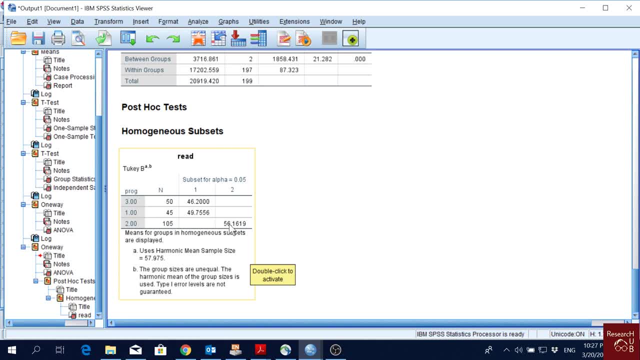 subset, which means there is a significant difference between group two and one and group two and three. okay, so that's what it means. and so what? what if we assumed equality of a non-equality, of variance? so we can also see that here. we'll see that we'll actually get the same result. so i go to postdoc again. i'm taking this. 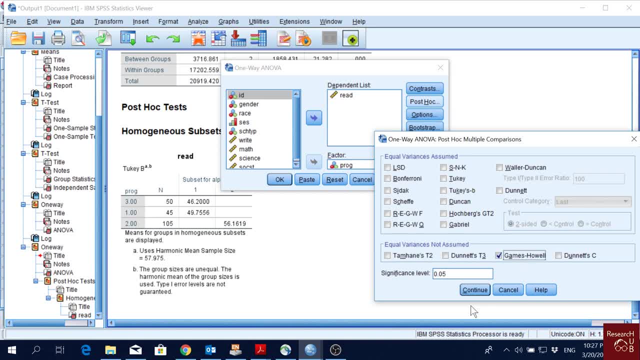 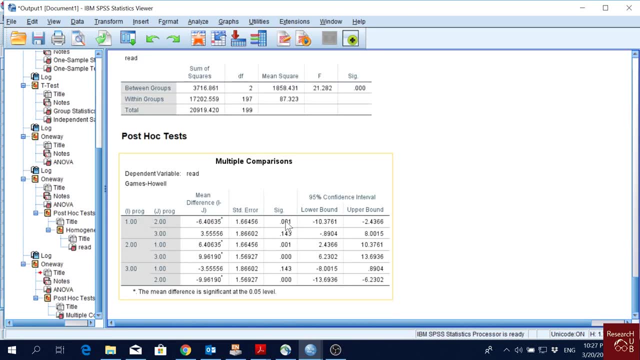 and i'm, let's say i'm going for this one games whole will okay, continue and okay. so here again you will see that the significance. here there is a significant difference between group one and group two, but not with group one and group three. okay, again, we'll. 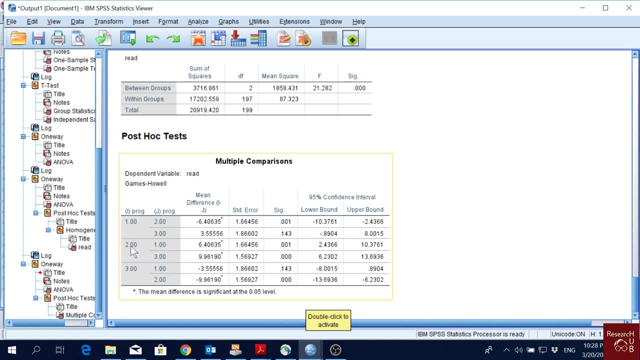 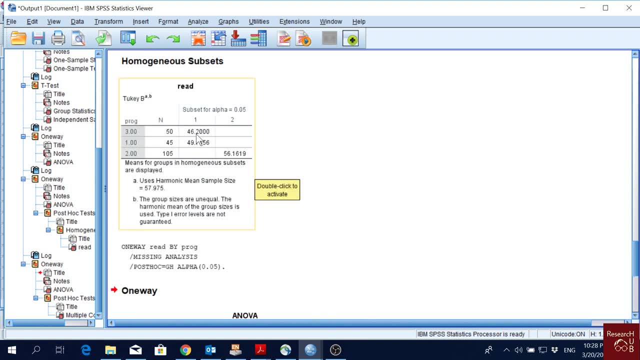 group two and one, but not between. no, yeah, again, group two and one and group two and three, but not with group one and three. okay, if you remember, like in the previous case we had group one and three in the same group, so they were not significantly different from each other, but again, similar to. 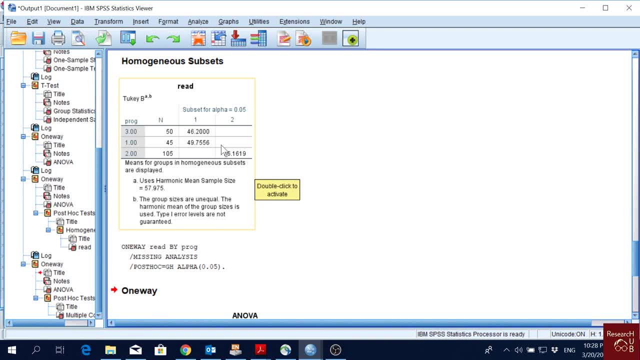 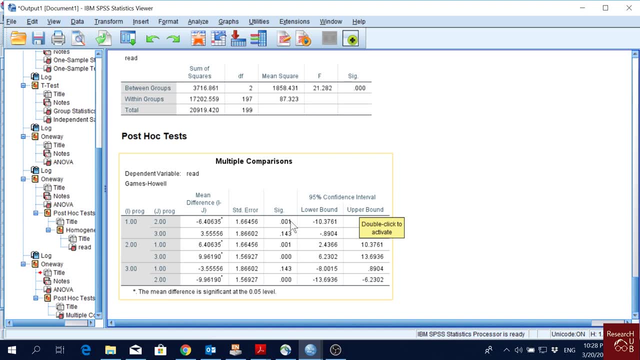 that we we have group one and there's a difference between one and two and one and uh and two and three. okay, these are the difference ones which we see here as well. so, yeah, the significance values here are the significant differences. we also have accordingly, the confidence intervals, lower bounds and upper bounds for the differences. 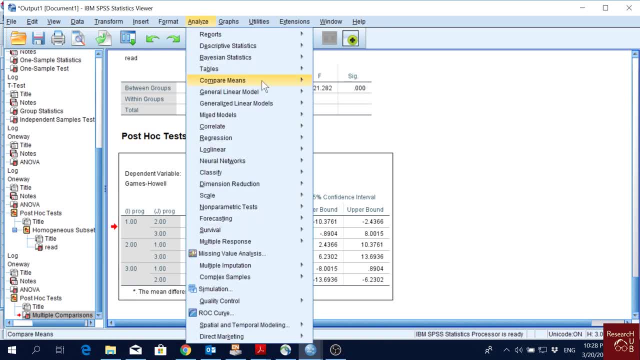 yeah, that's what we have here. but now, let's say we had some, some situation where we had collected data from one group of people multiple times. okay, so i have, i have color, i have students have done the reading reading test in 2018 and again in 2019 and i want to see. 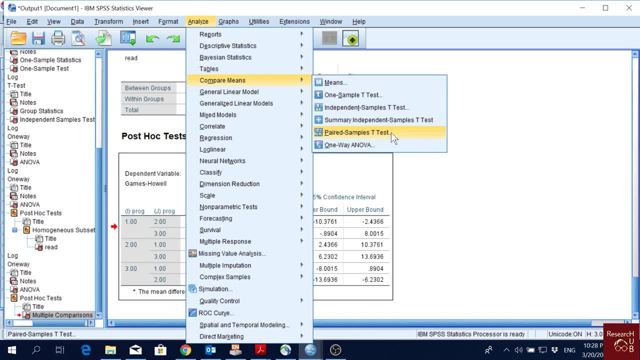 if there is a significant difference in the reading score of 2019 and 2018 of the same students. in such cases, when we collect data repeatedly from the same sample, we have to use paired sample t-test. in those cases we cannot use the others one. 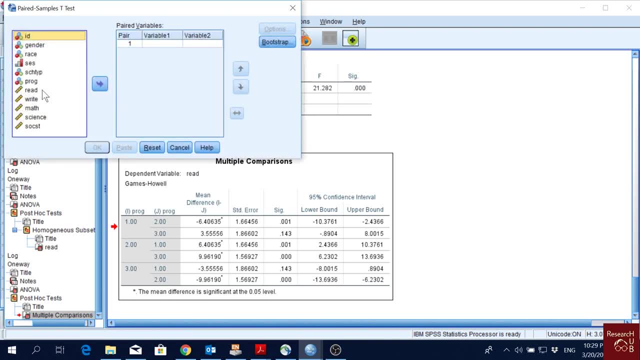 okay, so we'll click here, but down with the problem is that we do not really have any variable: which. which represents? uh, which represents repeated measures. but just to show you, i'll just pick reading, and i'm assuming that writing is my reading score in 2019. it's just, i'm. 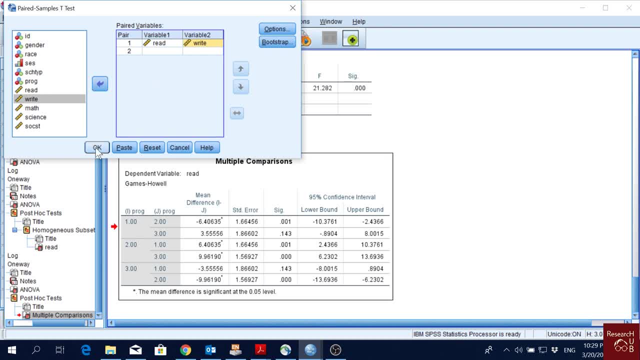 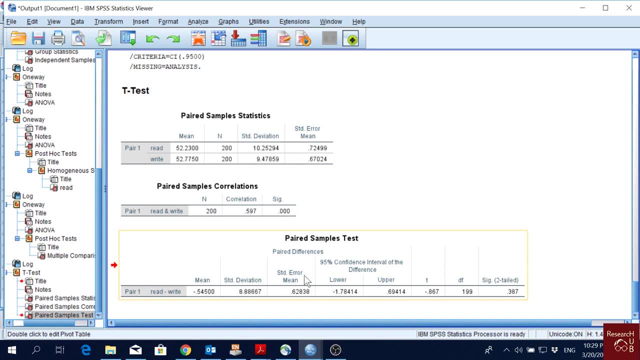 assuming now, okay, it's just to show you how it works, then i'll click ok and this is the result that we will get. so the differences in the mean and standard deviation, standard error. we will again get the confidence intervals accordingly and the t value is very low.